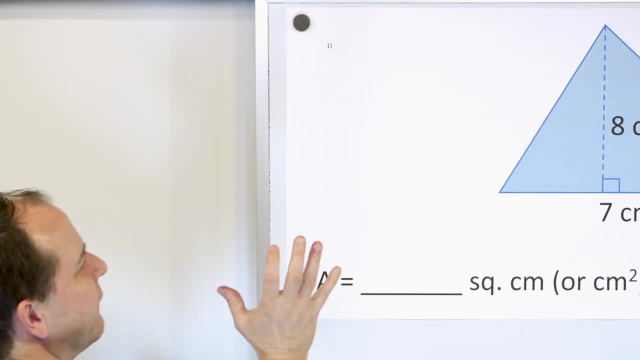 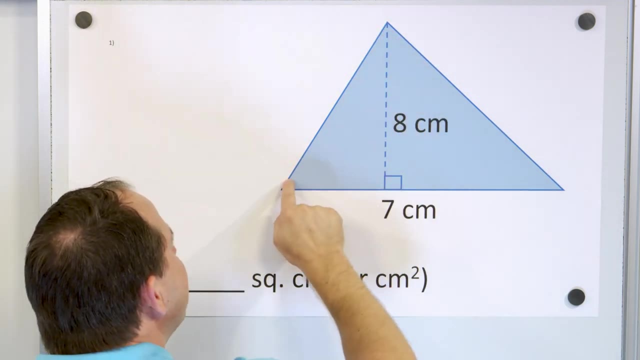 So let's go ahead, and before we solve our first problem, I mean our. actually, our first problem is going to be to find the area of a triangle like this where we have a base and a height here, but the angles in the corner they're not 90 degree angles. This one is because it's a 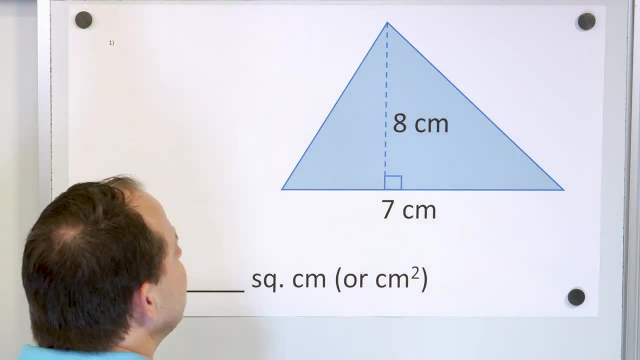 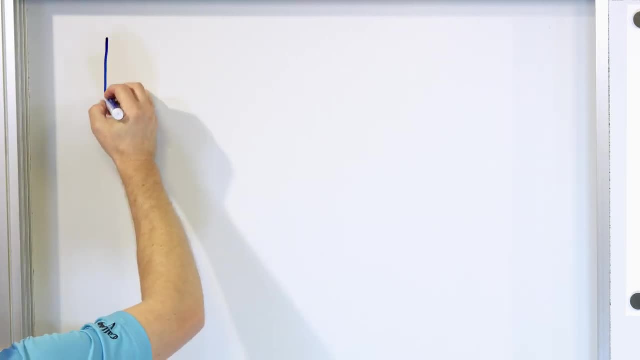 the height of this thing coming down, but the angles in the corners are not right angles there. So that's what we're going to be doing, But let's, before we do that, let's just take a trip down memory lane And let's talk about a couple of things. Let's first talk about a rectangle. This is a rectangle. 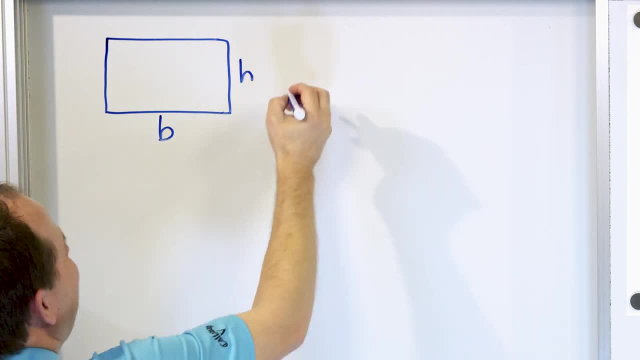 right. It has a base B and a height H. What is the area of this guy? the area of a rectangle? It's just the length times the width, But in this case it's the length is, or one side is B and one side is H, So it's base times height. the area of the rectangle is base. 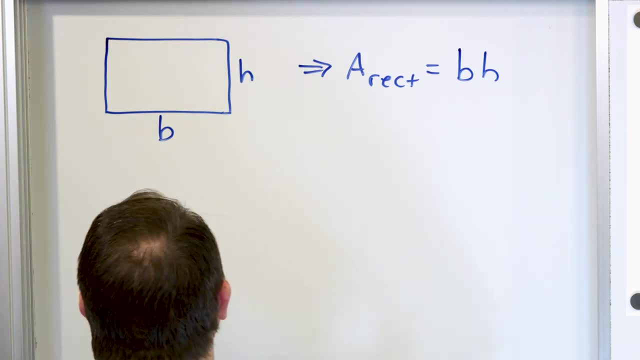 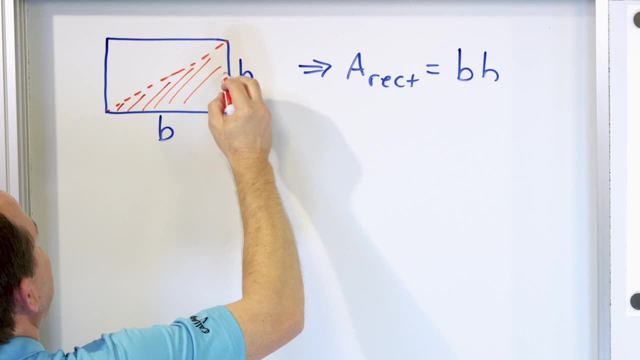 times height, right? So then if we say, instead of that rectangle, what happens if we cut that guy in half? we just literally slice it corner to corner And then we're going to find the area of just one of these halves of that rectangle which look 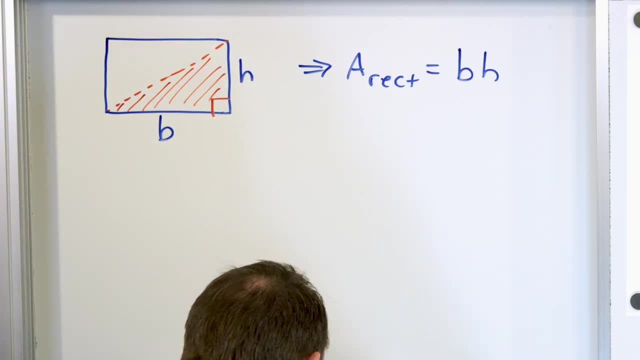 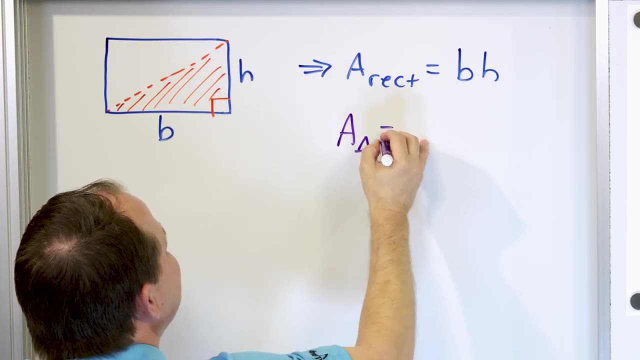 forms a right triangle. This is a right triangle here. So from this diagram you can see that if the area of the entire thing is just base times height, then the area of the right triangle which is inside is just one half times base times height, because you would take the whole area and 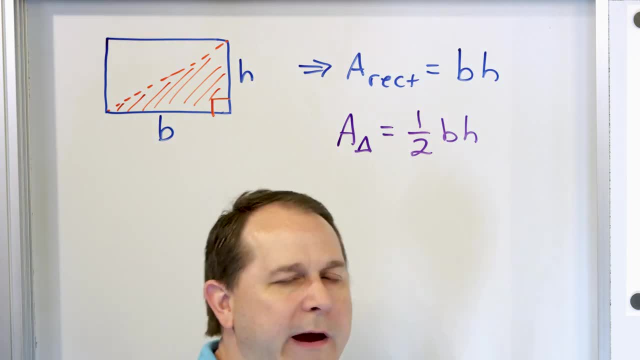 you would just cut it in half, divided by two. That is where the area of the right triangle comes from. One half times base times height comes from taking the area of the rectangle- if you made it into a rectangle- and just cutting the thing in half. That's where that comes from. 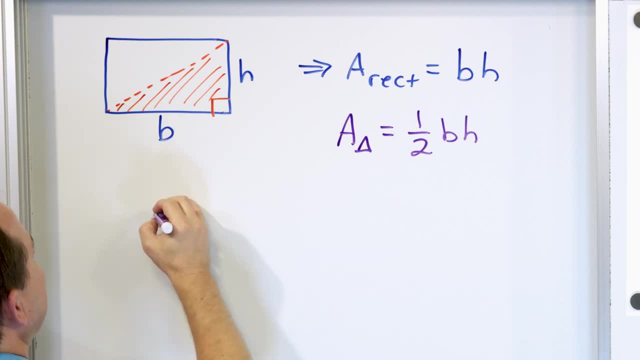 But now let's take it a step further. So this type of triangle would be- I guess I'll just draw it here- a right triangle like this, with a base and a height. That is where this area equation is applied to. But let's change it a little bit. Let's change it Instead of a right triangle like 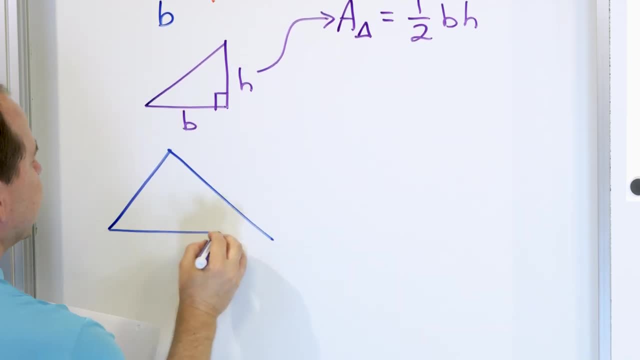 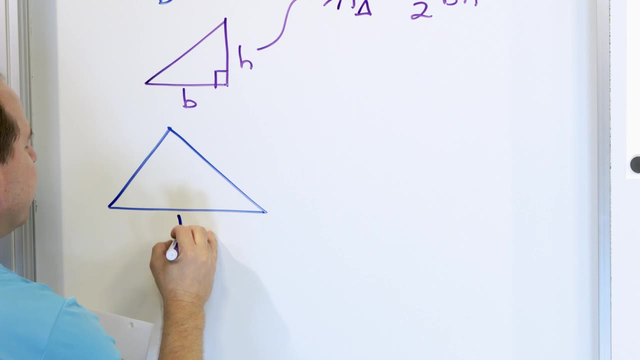 that let's make it a more general triangle shape, something like this, right? Notice, this is not a right angle in any of the corners, but we can still say that it has some sort of base to it And it has some height. right, You can measure the height from the side here, the tippy top. 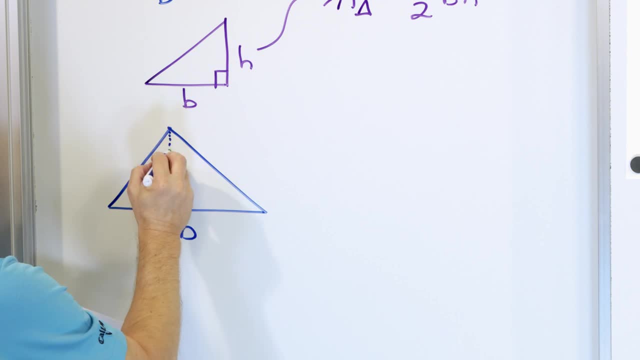 down to the bottom. That would be the height of this thing. Or, more generally, what you would usually do is you would put H down here And you would draw a little right angle, telling yourself that as you drop the line to the bottom there, it's going to make a right angle there And the 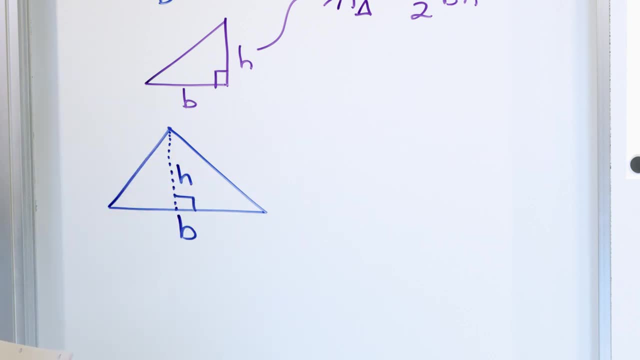 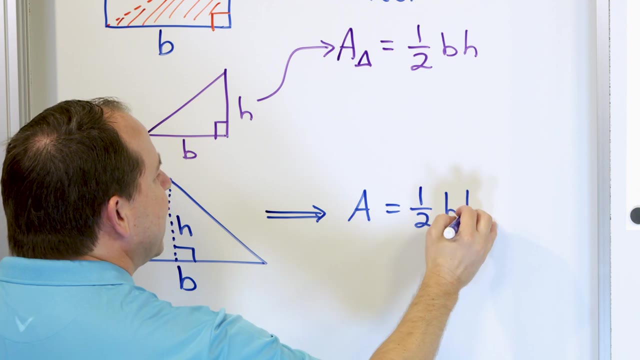 height from the base all the way up to the tippy top is what we call H. Now it turns out that the area of this triangle is going to be a little bit smaller than the base. So let's say that this triangle is exactly the same equation: one half times the base, times the height. So you see. 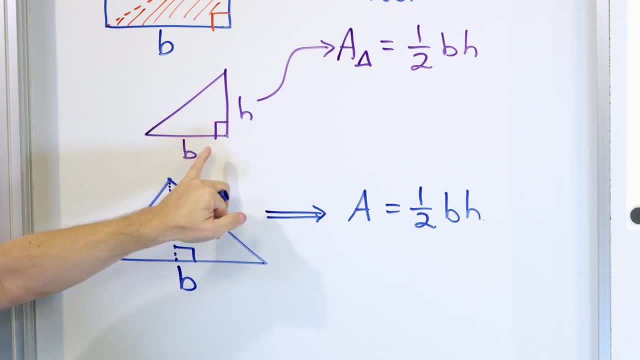 it's no different. There's no different equation Here. it's just a little easier to visualize because I can show you in terms of the rectangle: the area of this guy is one half times the base, times the height, which is what we got for the right triangle. But what I'm telling you now is: 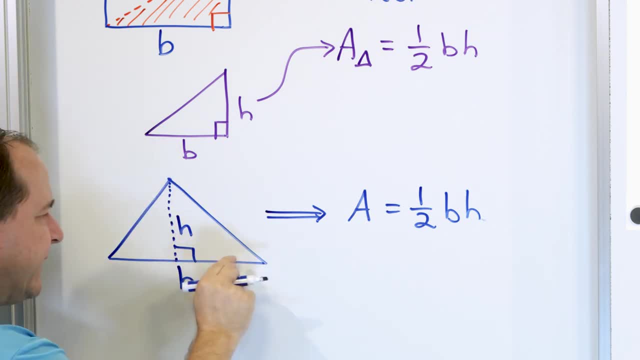 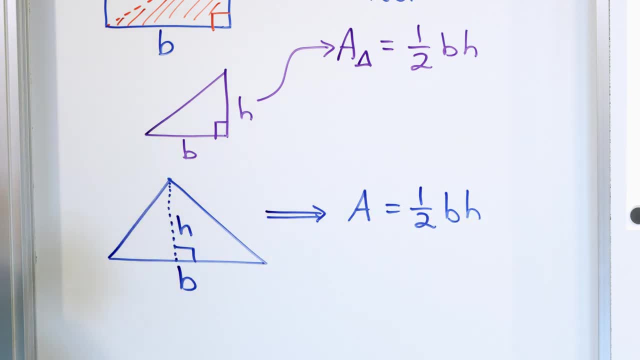 this distance one half times base times. height is exactly the same thing And you could prove that to yourself. I'm not going to do it here, But you see, when you cut it like this, you form a right triangle right here and you form a right triangle from here. So you could write down what. 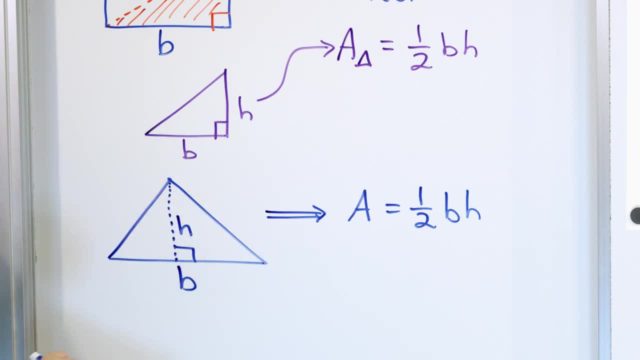 the area of this is and what the area of this is, And when you put it all together, you're going to find out that it's exactly the same equation as what we have been using all along. Now let me show you an equation of a really weird triangle. What about a triangle like this? Something like this: 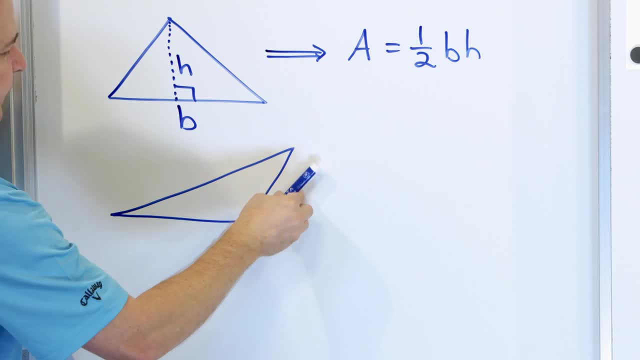 This does not look like a typical triangle, but it is a triangle because it has three sides right, But notice, it looks quite a bit different than this, than the other ones above. What would be the area of a weird looking triangle like that? Well, it still has a base here and it still has. 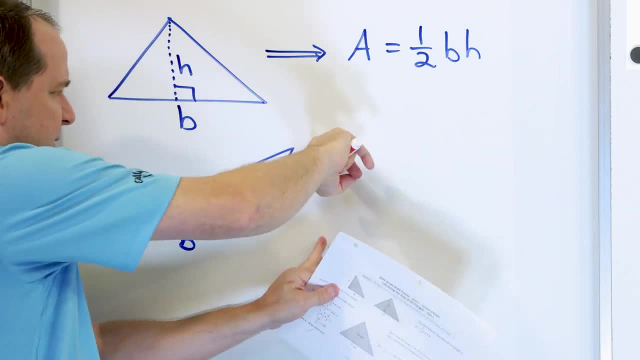 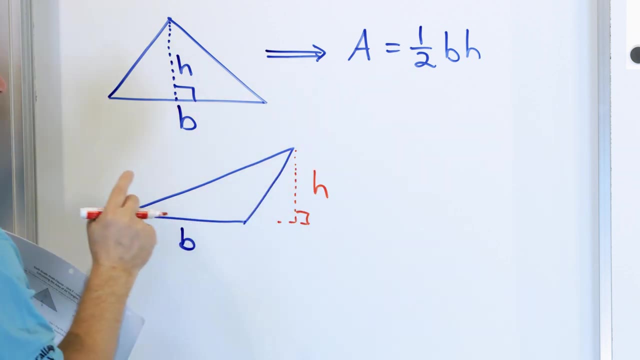 a height. I could measure a height by literally dropping a line down. You could just kind of drop a line down like this, I guess something like this, and call that h. So the height of this triangle is, from the very base all the way measured to the tippy top. Same definition. 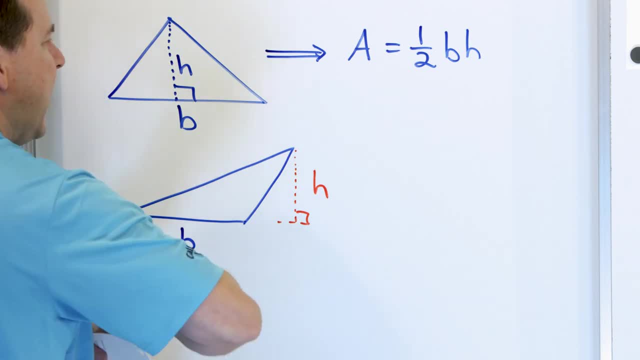 here, And we call that a distance h right. And so what do you think the area of this thing is going to be? It's going to be one half times the base, times the height, again And again we could calculate this, We could draw this as a larger triangle and then this forms a right. 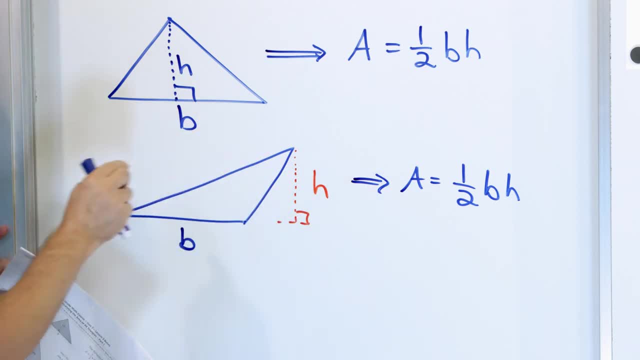 triangle here. We could subtract this area out to tell us what this area is. I'm telling you that there are ways to go and figure out and show yourself that this is the actual equation of the area of this thing, by looking at the area of the whole thing and subtracting out this little. 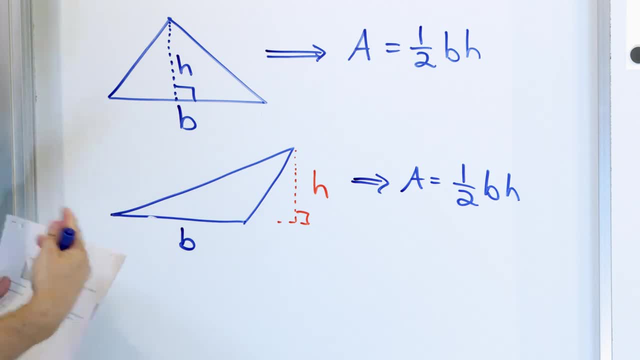 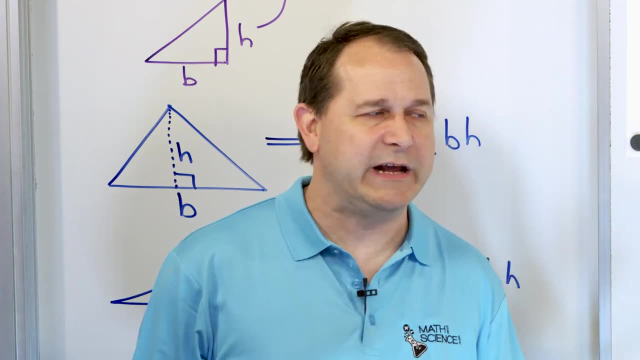 piece here, And we could do the same thing with all these other ones. But the bottom line is we don't really need to do any of that stuff, because it all works out that the equation of a triangle is the same for all triangles. That's basically what it is: One half times base times height. 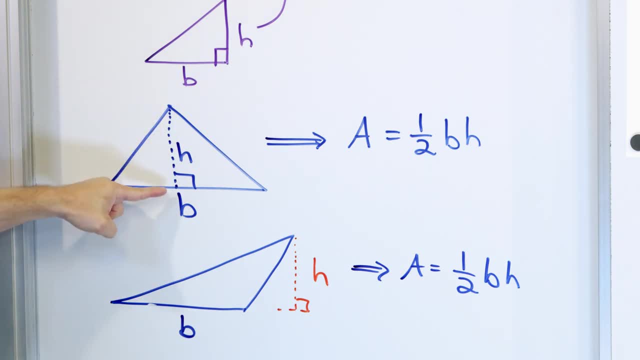 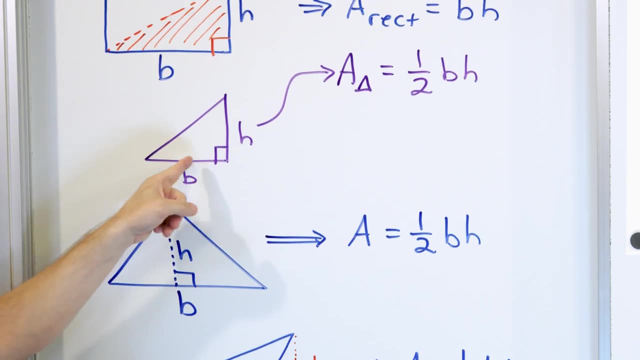 It's just that when you have a triangle like this, you measure the height from the top all the way down. When you have a triangle like this, you measure the height from the top all the way down- level with the base here- And, of course, if it's a right triangle, we measure it the same way. So 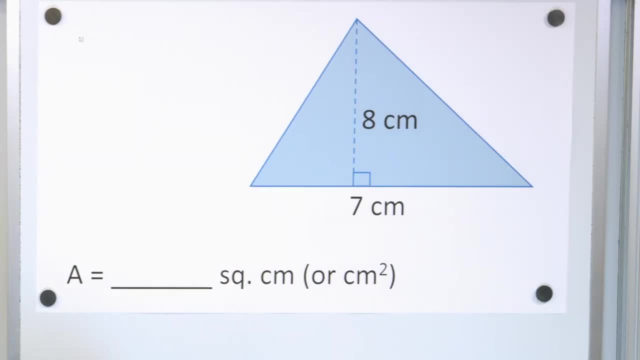 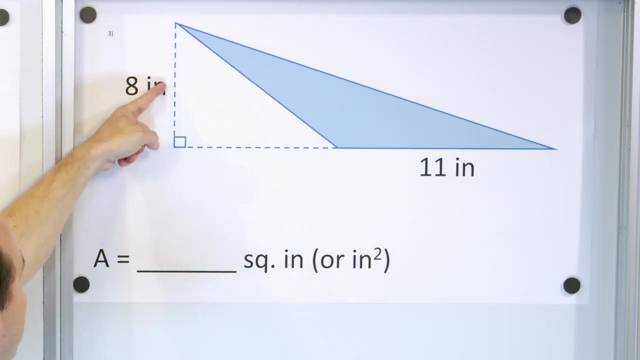 exactly the same equation in all three cases. So we're going to solve problems like this, Problems like this And also problems like this. Notice, the height here is measured from the top all the way down to the base, But we're defining the area of the shaded region in blue, So let's 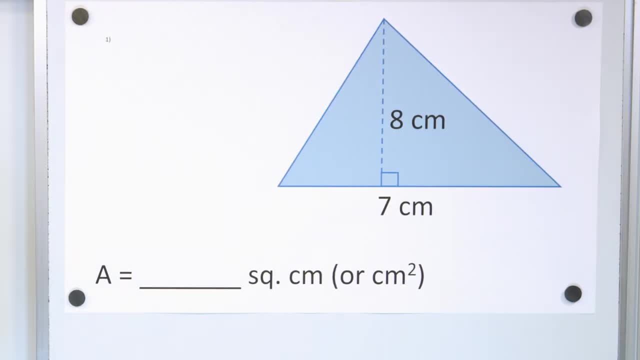 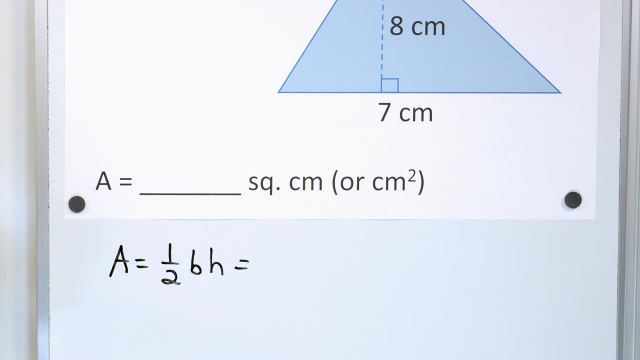 go ahead and apply that and calculate the area of these guys. What would be the area of this triangle? You only have to remember one equation: One half times the base times the height. You're going to use it over and over again. So what do we have? One half times the base, which is seven. 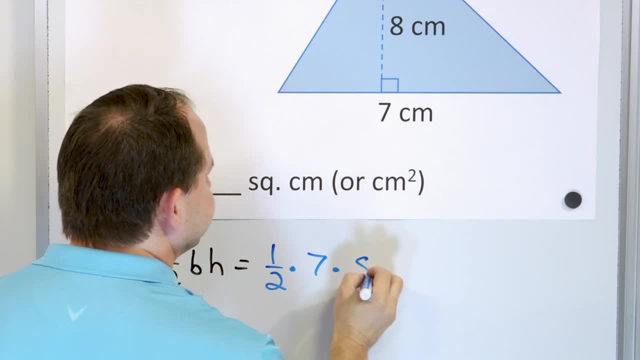 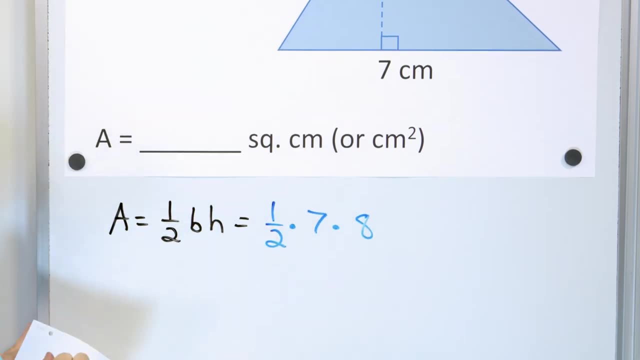 times the height, which is eight Right One half times seven times eight. Now you can do it any way you want. You can write these as fractions and multiply the tops and multiply the bottoms. You can multiply them in any order you want, because you're going to get the same. 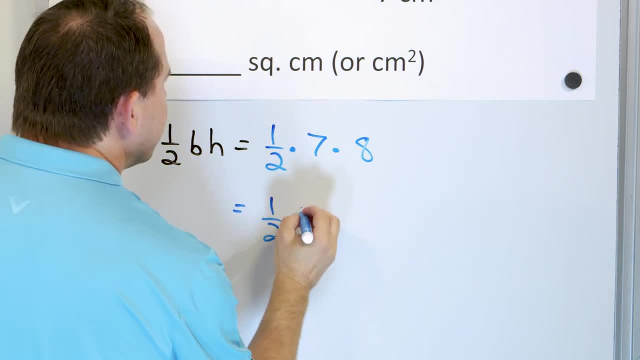 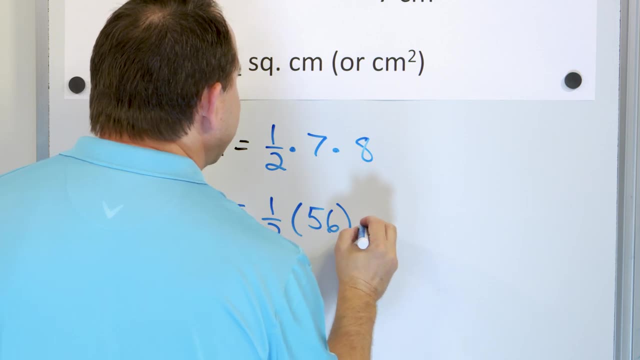 answer. What I'm going to do is multiply One half times. I'll multiply these Seven times eight, I know, is 56, right? So what I'm going to have is 56 over two, right, Because you can say this is over. 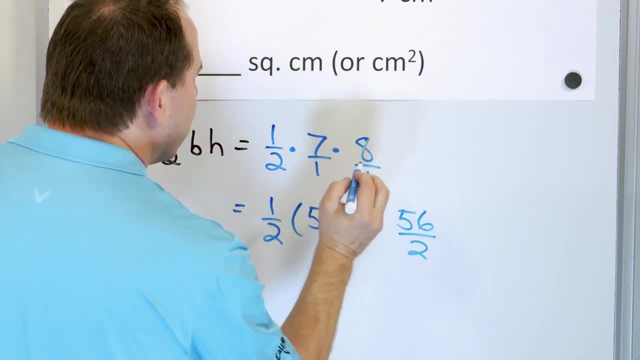 one. this is over 3, this is over 1, right, So I'm going to have this as the part of my set. I'm going one this is over one, so this 56 will be over one. Multiply these two and get 56. Multiply. 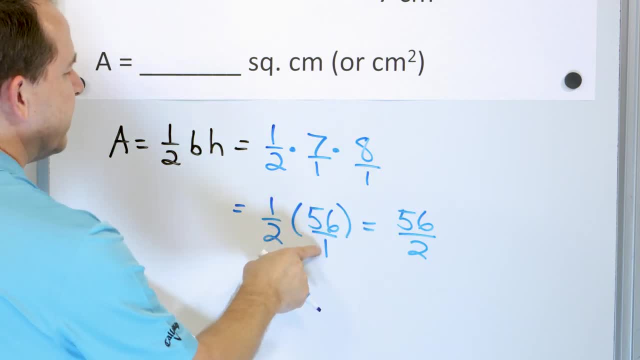 the ones to get this. You're going to multiply this to get 56.. Multiply this to get two. So, ultimately, what you have to do is take 56 and cut it in half. What is 56 divided by two? Now, I'm not going to do it for every problem, but you can say 56 divided by two. 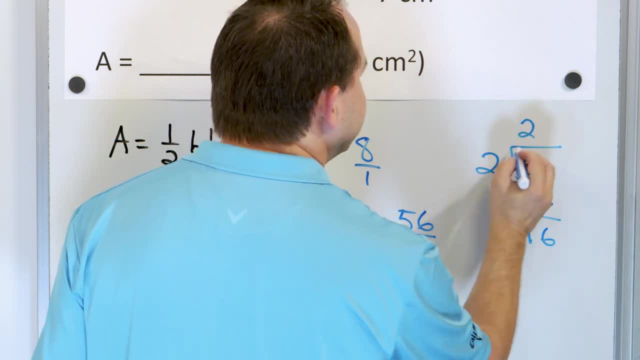 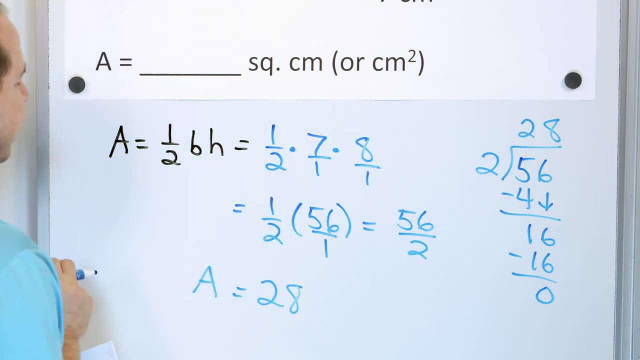 Two times two is four. Get a one. Drag down a six: Two times eight is 16.. Remainder: zero. So you get an answer of 28.. The area is 28.. And what is the unit? Centimeters times centimeters. 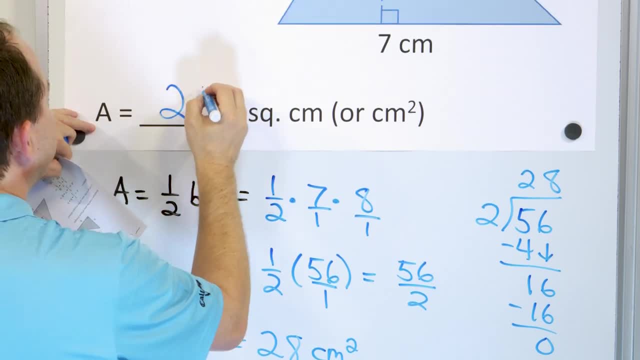 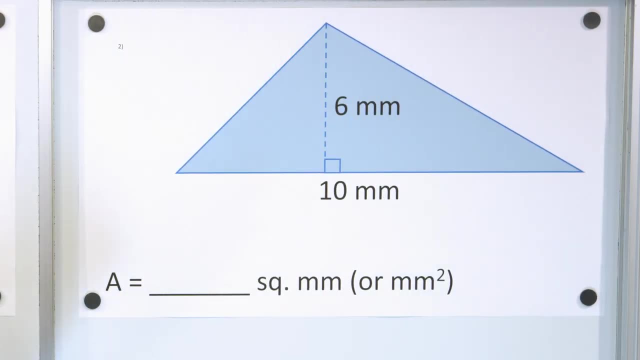 is centimeters squared or square centimeters, So we're going to call it 28 square centimeters. The point of it is for you to know that the equation of the area of a triangle is the same, really, for all triangles. It's just we start with right triangles because they're 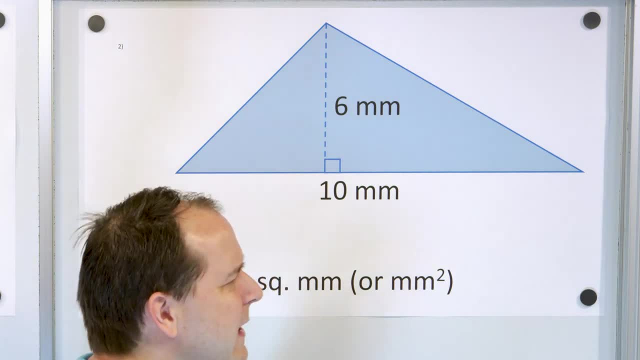 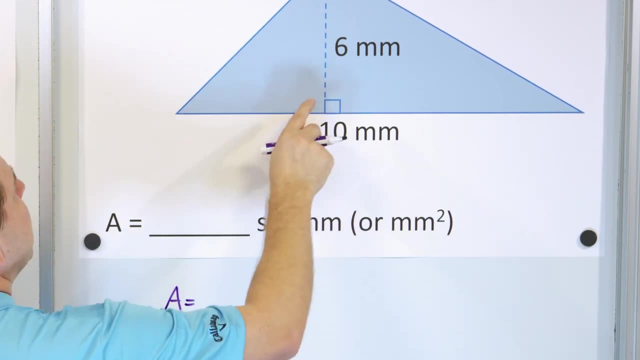 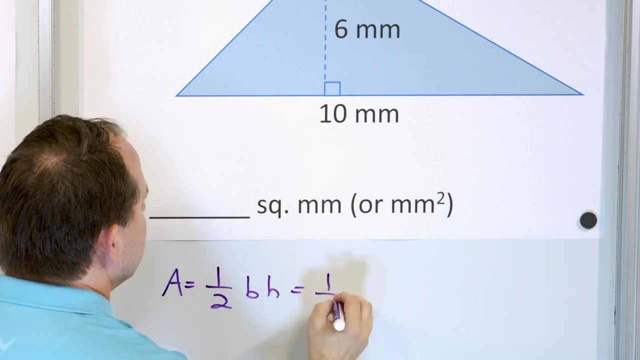 easier to understand and now we're opening it up to different shape triangles or different types of triangles. Let's take a look at the following triangle: Six millimeters, ten millimeters. Equation is the same: One half times the base times the height. So one half times the base is. 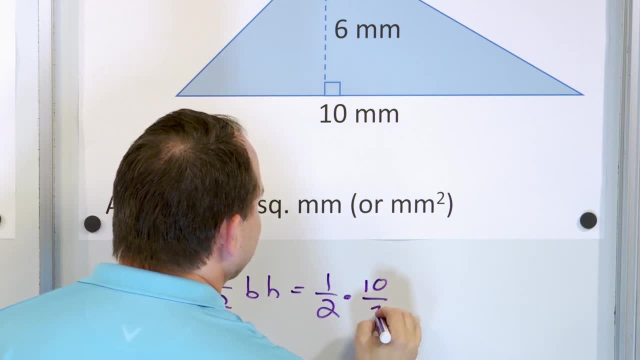 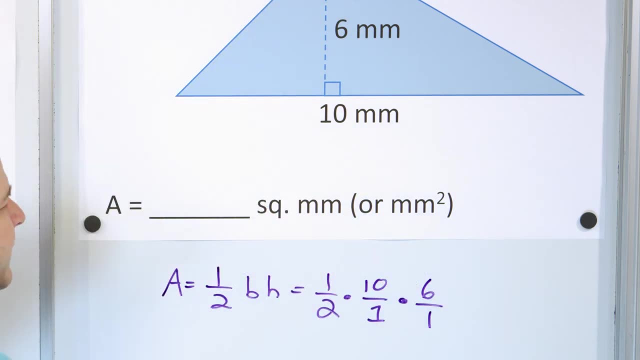 ten, So we'll be multiplying times ten. I'm going to write it as ten over one, though, And then the height is six, Multiply by six. I'm going to write that as six over one, So I'm multiplying by ten, multiplying by six. So one times ten is ten. Two times one is. 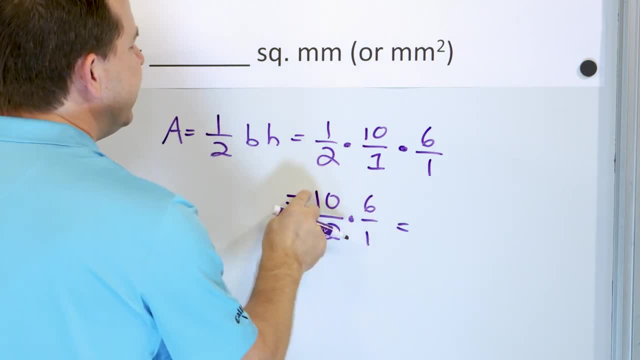 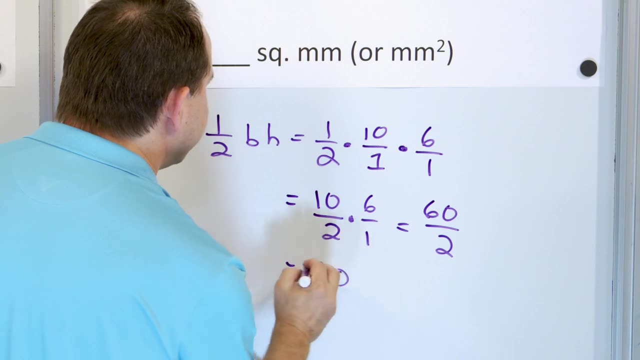 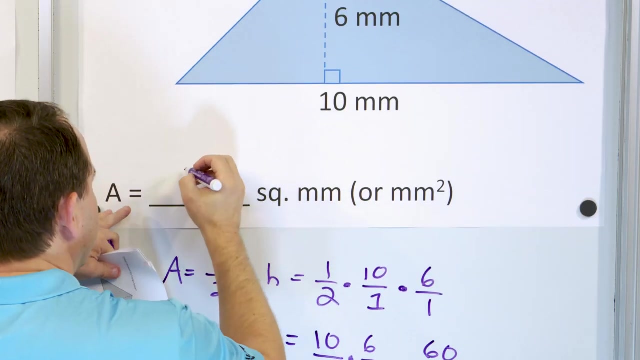 two. So we'll have to multiply by the six over one. Ten times six is sixty, And two times one is two, And sixty divided by two is thirty, And so that means the area is thirty. what It's millimeters times millimeters, which is millimeters squared, So it would be thirty. 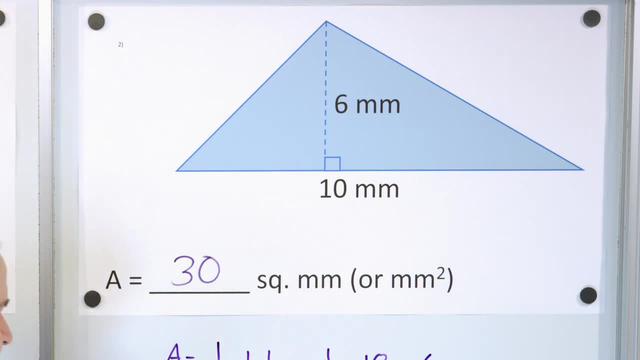 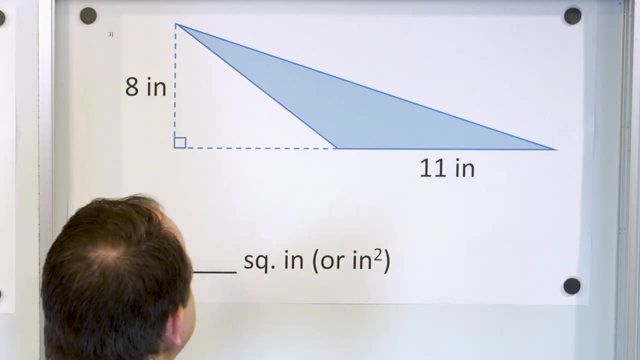 millimeters, squared or square millimeters, However you want to say it. All right. Now, here is the oddball type of rectangle or triangle, But it's the same thing. You want to find the area of the shaded region in blue right here. So we have to identify. 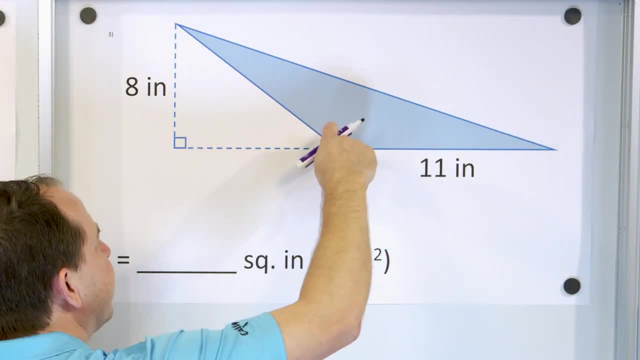 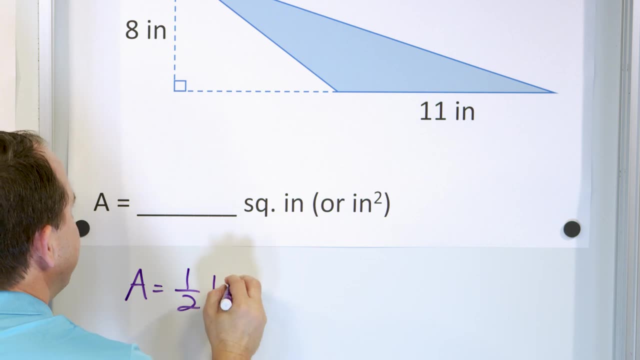 the base- The base is eleven- And identify the height, which is the distance from this base all the way up to the tippy top measured here as being eight. So the area is again one half times the base times the height. The base is eleven. So I'm going to write. 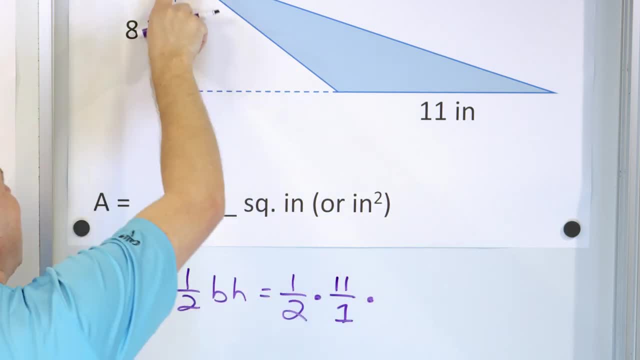 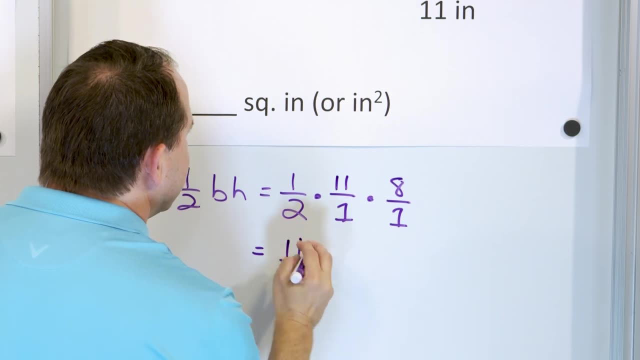 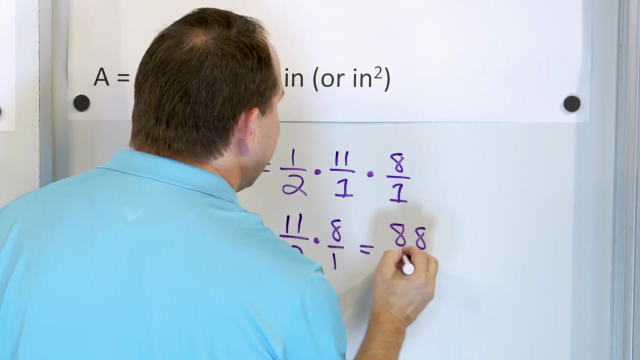 that as eleven over one, And the height is eight. So I'm multiplying by eight. I'm going to write that as eight over one. All right, So let's multiply. One times eleven is eleven. One is two. Still have to multiply by the eight over one. Eleven times eight is eighty-eight. 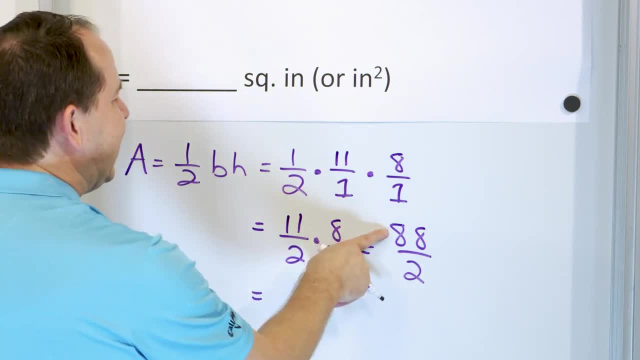 And two times one is two. Now you can do the long division on eighty-eight divided by two. But I think you can convince yourself: when you divide each of them by two you'll get forty-four, And so the area here is forty-four, And the unit is inches times inches, which. 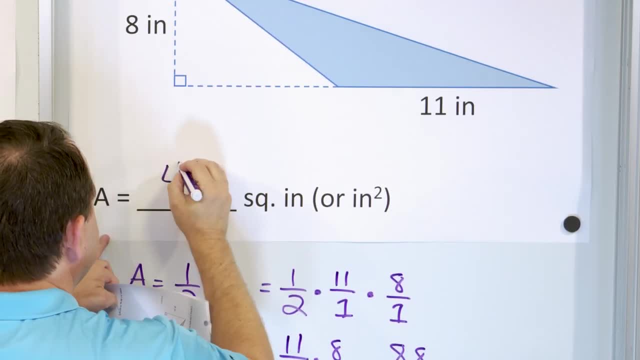 is square inches, Or inches squared, However you want to say it. So forty-four square inches, All right. So I'd like you to solve these yourself. I'm going to take these three down. We have two square inches. We have two square inches. We have two square inches. We have. 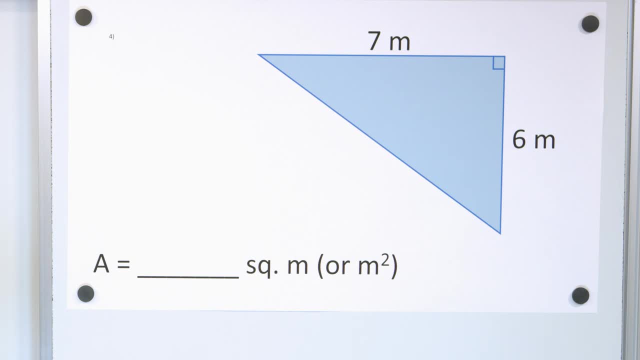 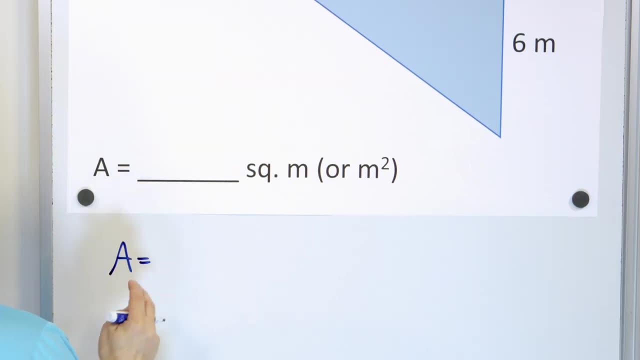 two more, And then we will be complete with this lesson. All right, Next problem: Let's take a look at this triangle. here We have six meters and seven meters. The area of this guy And this particular one actually happens to be a right triangle. You see it in the. 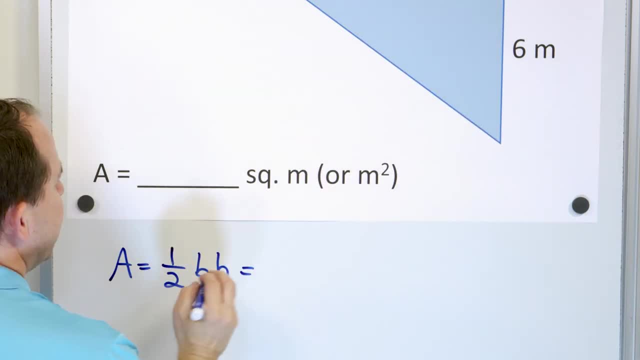 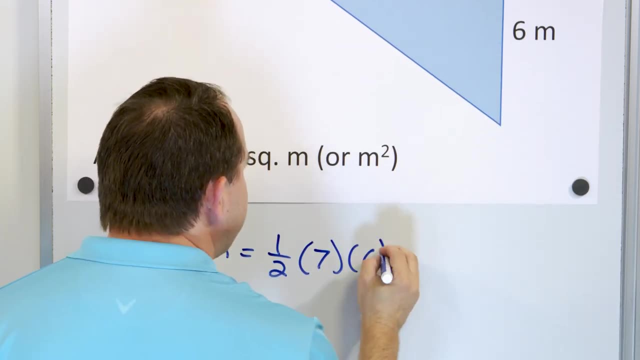 corner there Is one half times the base times the height, So it's going to be one half times seven times six. Now I could write these as fractions and do it the other way, But I'm trying to show you some variety here. I don't really want to do one half times the base. 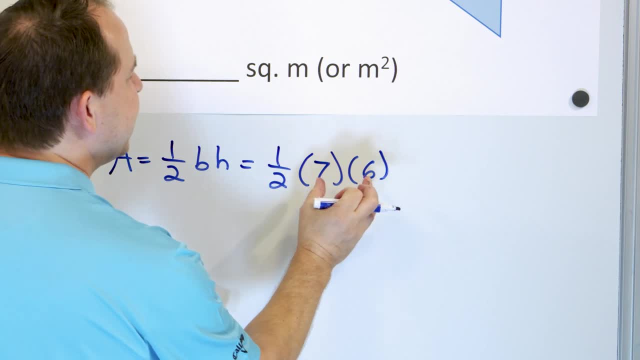 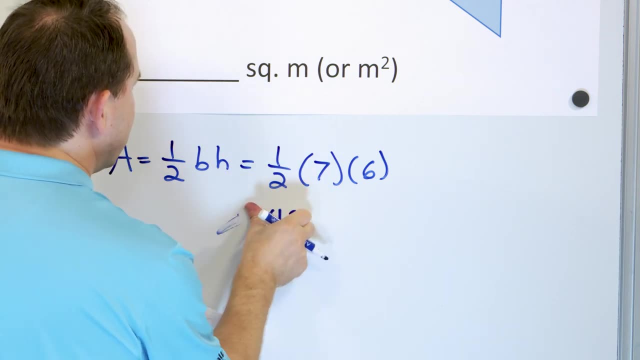 I want to do one half times seven, because I know that that's going to give me a decimal answer. So instead let's multiply this: Seven times six is forty-two, So it's one. Well, I guess it's forty-two. And then what I'll do over here is I'll say it's one half times. 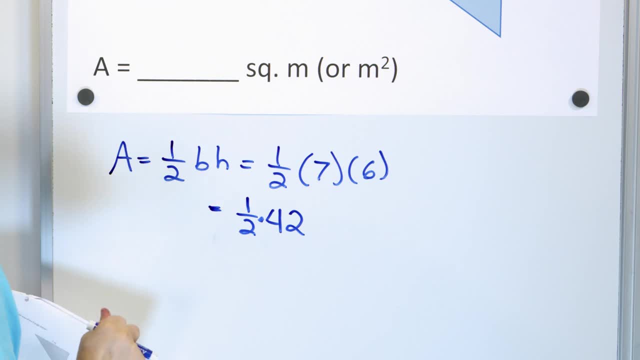 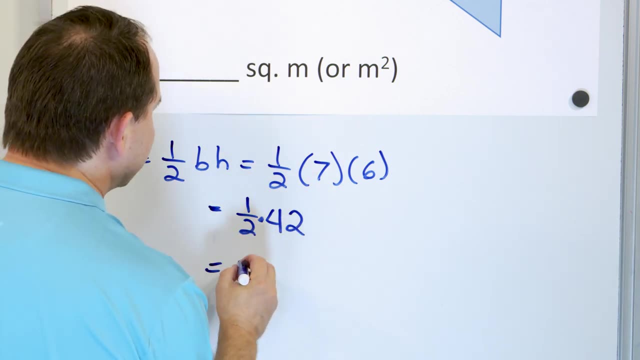 forty-two, One half times forty-two. So in other words, one half times forty-two is the same thing as taking forty-two and dividing it by two. Right, Forty-two divided by two is going to be twenty-one. You can see that when you divide this by two and divide this, 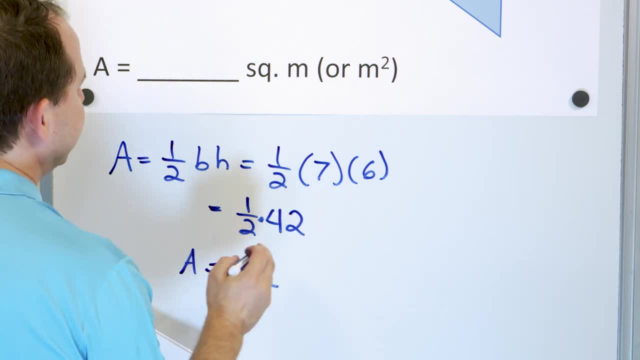 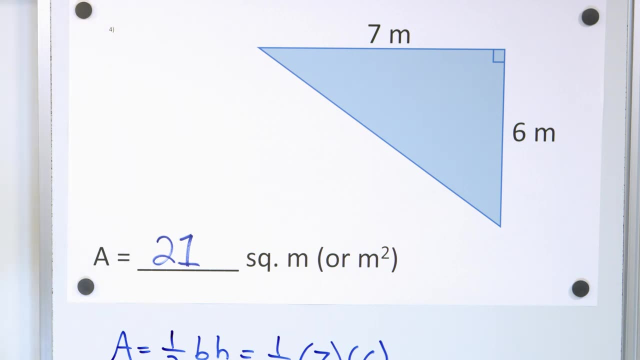 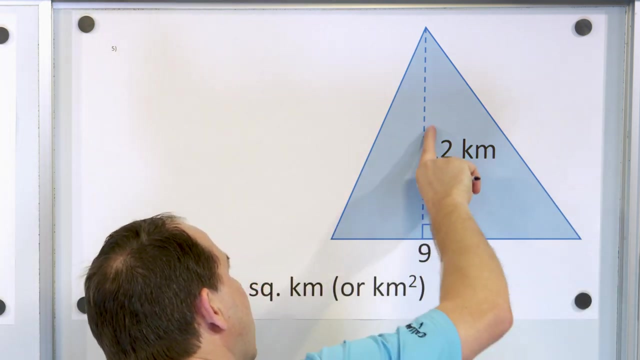 by two, It's going to exactly equal Twenty-one, So the area is twenty-one meters squared. Twenty-one square meters, also known as meters squared. Alright, here's our very last triangle that we have. Nine kilometer base, Twelve kilometer height. The area of this guy is one half times the base times. 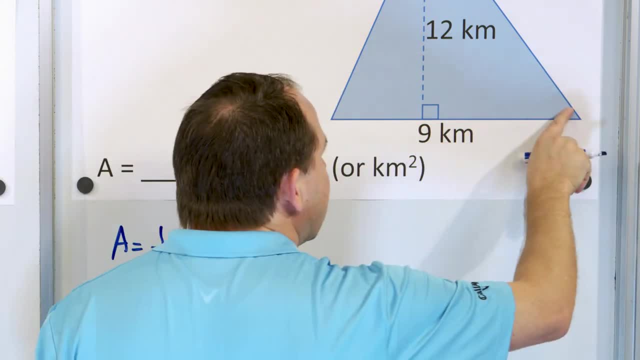 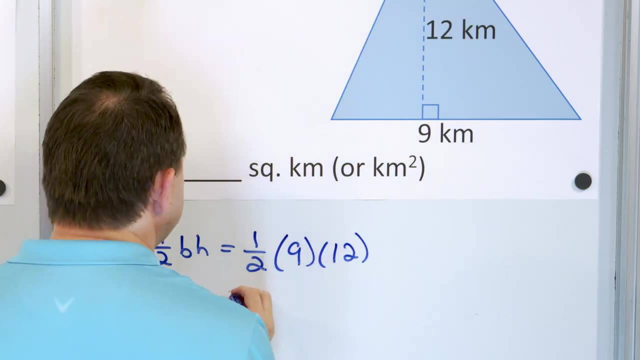 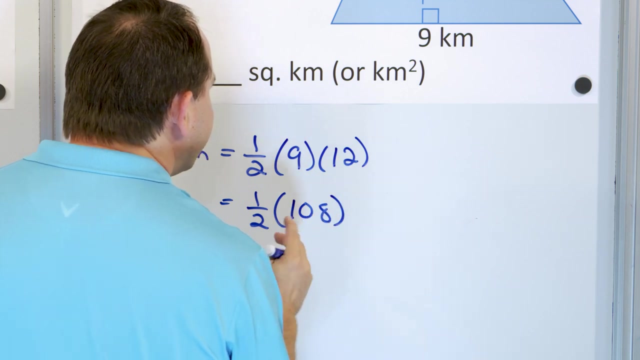 the height, One half times the base of nine and times the height there. So the base is nine and the height is twelve. Right, So one half times What is nine times twelve, It actually works out to be, when you multiply this out, a hundred and eight. So what you have to do is basically what you.